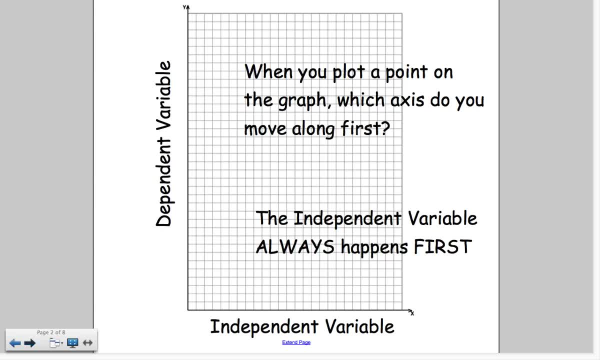 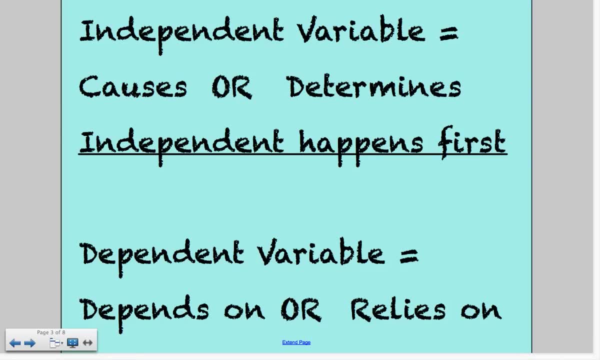 always happens first. So let's take a look at what that means in a situation. here We have the independent variable, which is causing or determining what happens to the dependent variable. Now remember that the independent variable happens first. The dependent variable depends on or relies on that independent variable. Without the independent variable, the dependent variable can't do anything. Alright, 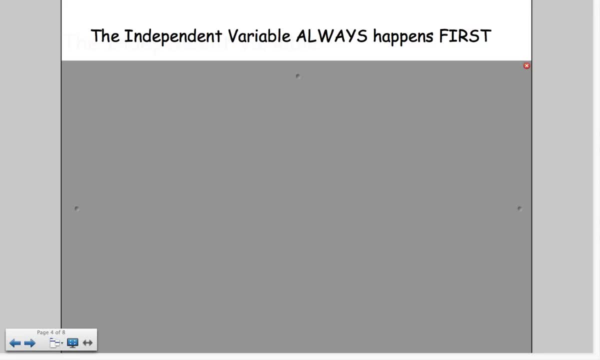 Remember this: The independent variable always happens first. So what we're going to do is we're going to find the independent variable by looking at a situation and figuring out what has to happen first before the other variable can happen. So here we go. We've got the number of cars sold and the price of the car. Now what we have is price and number of cars sold. These are the two variables. What I want us to think about is which has to happen first. So let's take a look at this. 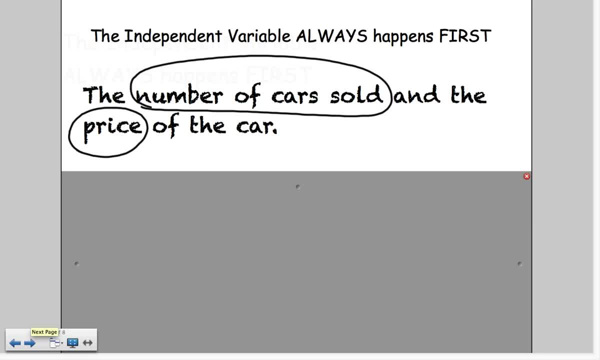 First, in order for the other one to even matter, or exist or happen. And what I want you to think about is: the first thing that's going to happen is the independent variable. Now, in this situation, if you don't price the car, there is no cars to, there are no cars to be sold, There is no number of cars that can be sold. So the price of the car is your independent variable because it has to happen first, Then the number of cars is the dependent variable. The reason 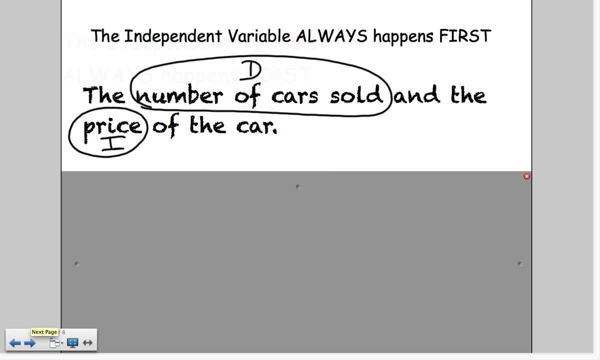 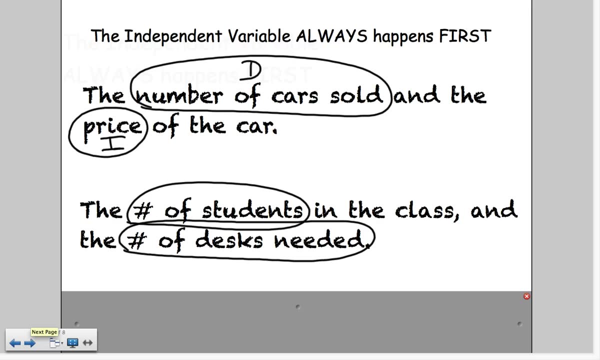 relationship here is: the higher the price, the fewer number of cars that are sold. The lower the price, the more number of cars that are sold. Alright, Here's another example: The number of students in class and the number of desks needed. Now, in this situation, again, we're going to be trying to find the independent variable first, which is: what do you have to have first in order for the other one to even matter or be affected? In this case, you have to have students. 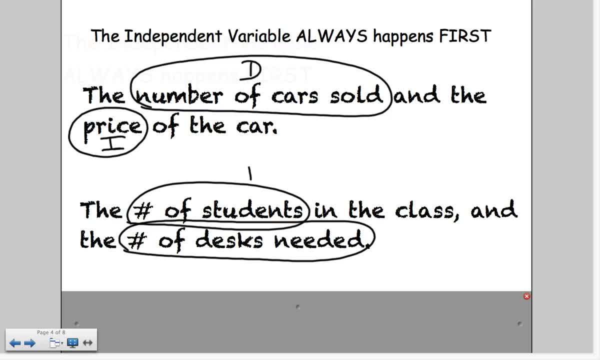 If you don't have students, there's no need for desks. So the independent variable is the number of students, making the dependent variable the number of desks needed. And this makes sense if you think about it, as the number of desks needed depends on the number of students you have. Now the relationship in this example is: the more students you have, the more desks you need. The fewer students you have, the less number of desks needed. Alright, let's do another example here. Remember the independent 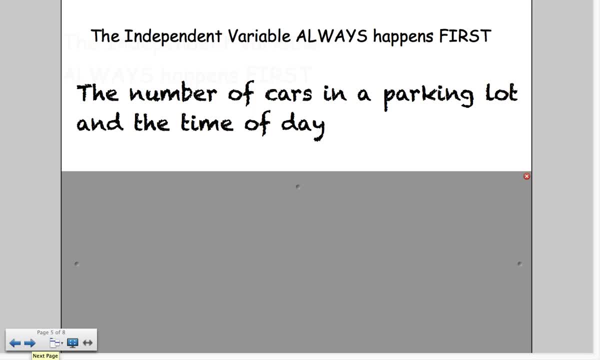 variable always happens first, Alright: The number of cars in a parking lot and the time of day. One variable is the number of cars, The other is the time of day. And think what has to happen first before the other variable is even important In this case. if you don't have time of day, you don't have cars. If there's no time of day, there really isn't anything else. So time of day is the independent variable and the number of cars. 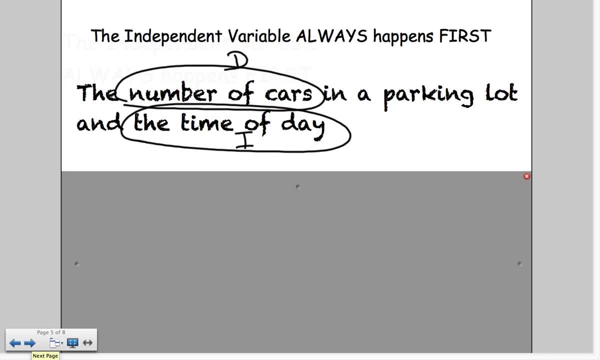 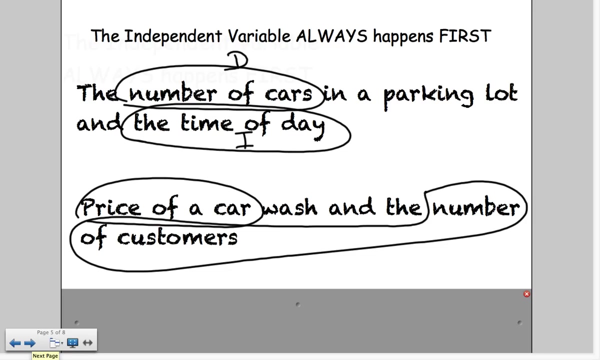 is the dependent variable, And that would make sense that the number of cars depends on the time of day. The relationship would be: if it's 2 am, there probably aren't very many cars in a parking lot. If it's 10 am, there's quite a few more cars. Alright, The price of a car wash and the number of customers. Again, what do you have to have first before the other variable even matters. If you don't have a price of a car wash, if you don't have the price set, there are no customers. 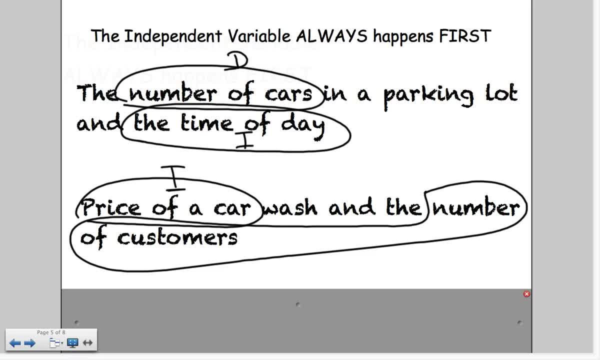 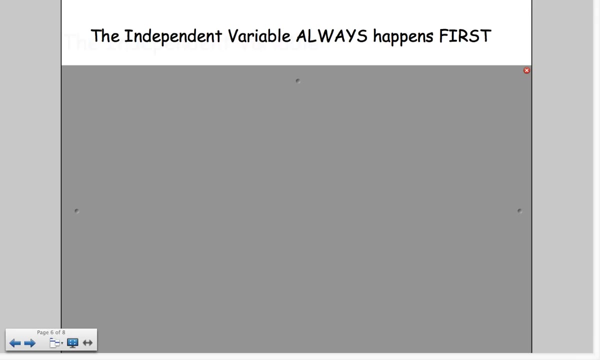 There's nothing that you're selling. So the price of the car wash is the independent variable and the number of customers is the dependent variable. And this actually makes sense. The number of customers depends on the price of the car wash. If you price the car wash too high, you won't get very many customers. If you price it lower, you'll get more customers. Alright, We're going to do more guys, because the more we practice this, the more permanent it'll make it. Alright Again, remember the independent. 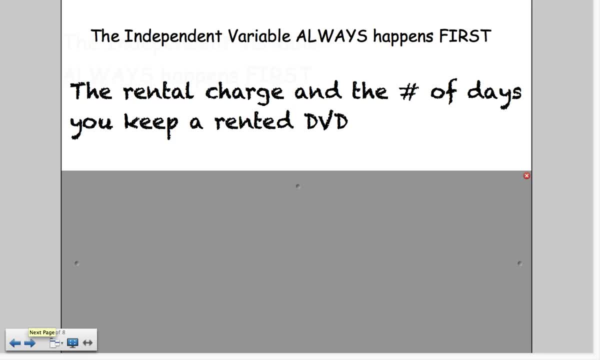 variable always happens first: The rental charge and the number of days you keep a rented DVD. We've got a rented charge, rental charge, and we've got number of days. Alright, If you think about it. what has to happen first? What, what needs to actually occur in order for there to be change happening to the other one? And in this case you have to have rented the movie for some number of days. If you don't rent this movie, there is no rental charge. So the rental charge depends on the number of days you keep a rented DVD. 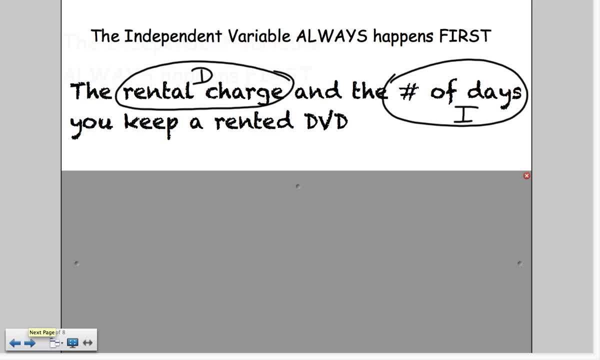 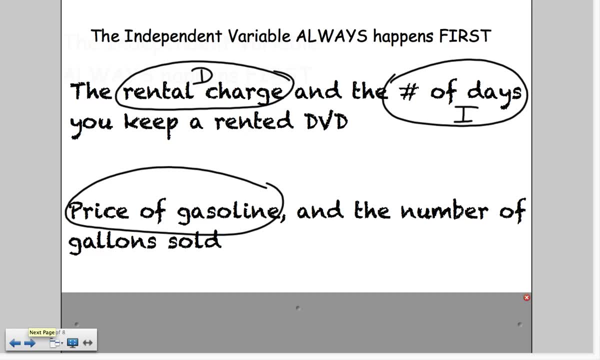 And in this situation here, the more days you keep it, the more the rental charge. the fewer days, the less the charge. Alright, Price of gasoline and the number of gallons sold: Alright, Think about it. What has to be happening first in order for change to happen in the other variable? Well, if you don't price gasoline, you're not selling gasoline. So the price of the gasoline is independent. It happens first. 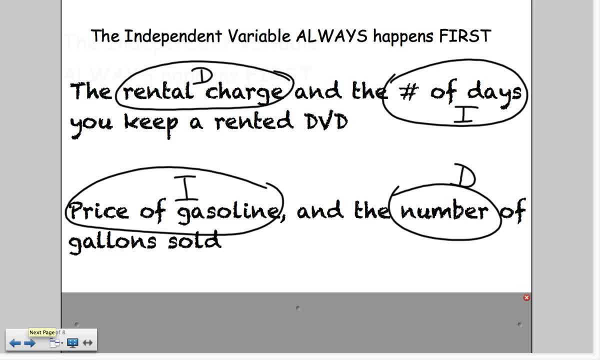 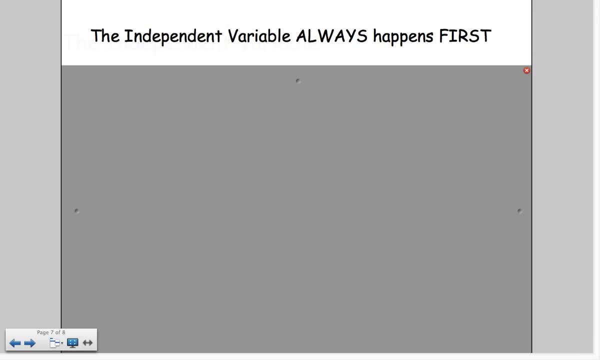 And it's what causes the number of gallons sold to actually happen. In this case, the relationship would be: the lower the price, the more number of gallons of gasoline sold, The higher the price, the fewer. Alright, We've got another one, another set of examples. here The independent variable always happens first: The price of popcorn at a theater. So price and the number of bags sold. These are two variables here. in this situation, What do you have to have first? 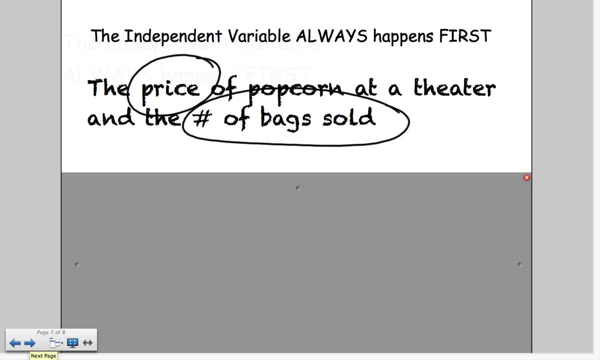 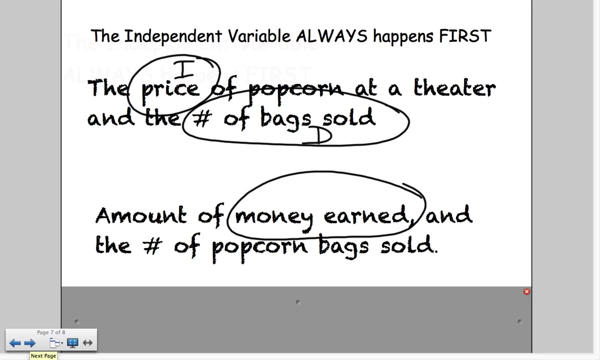